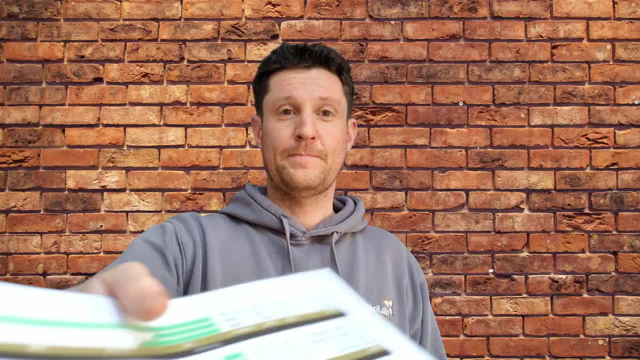 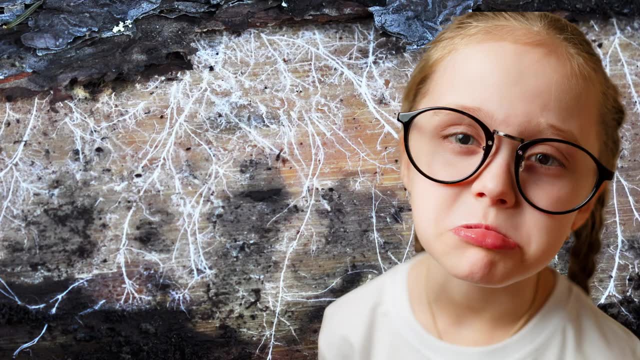 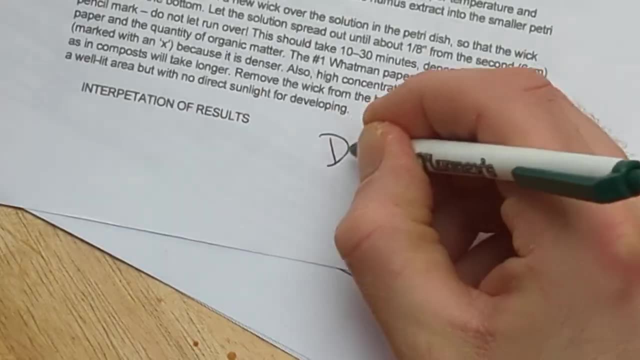 and the results would always be the same. Basically, their bacteria was all right or amazing, but the soil fungi was always lacking, And so we would send them off to do their homework. they'd maybe get a D, possibly a C plus, and we'd tell them they must try harder, which they duly. 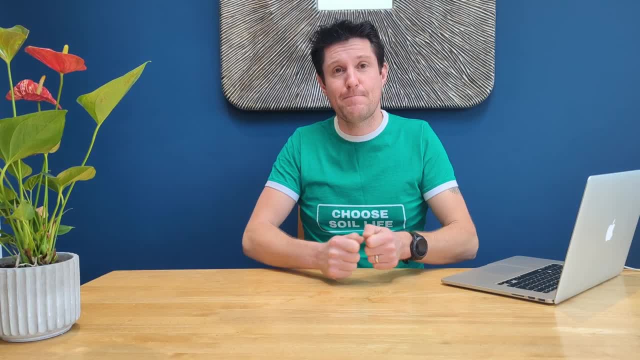 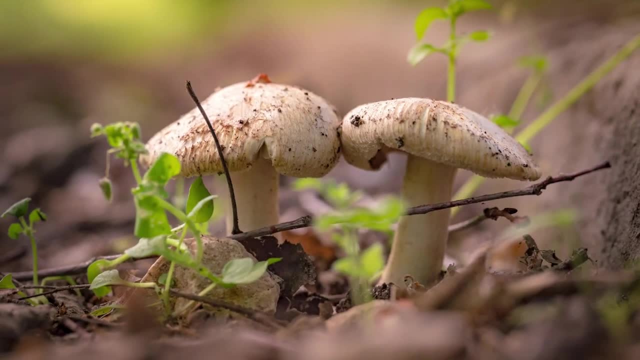 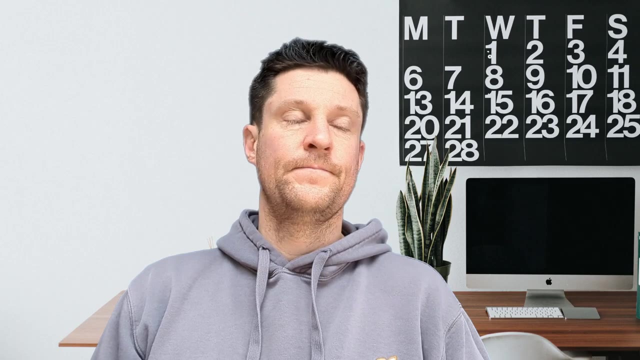 did Fair play to them. They would sit, plan things out, make changes and try really hard to increase their soil fungi And they would come back to us all excited so that we could test their soil again. And the results were the same: Soil fungi was still in short supply And they tried lots of. 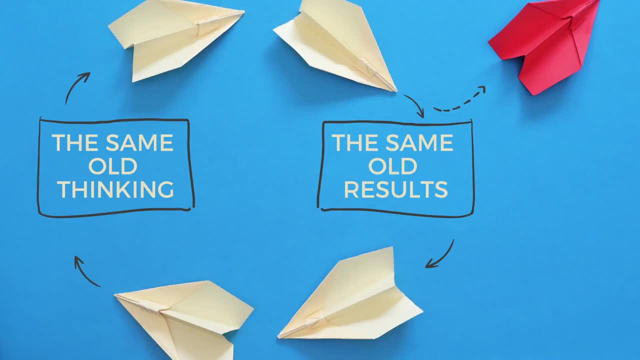 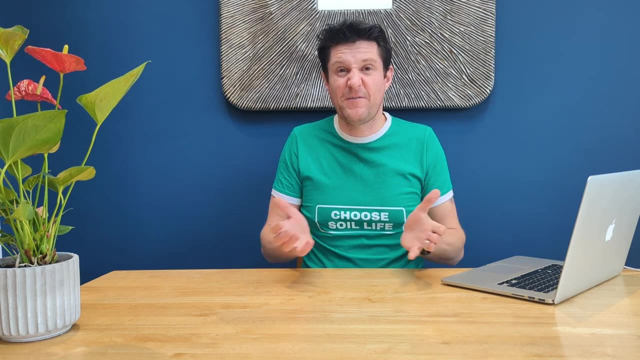 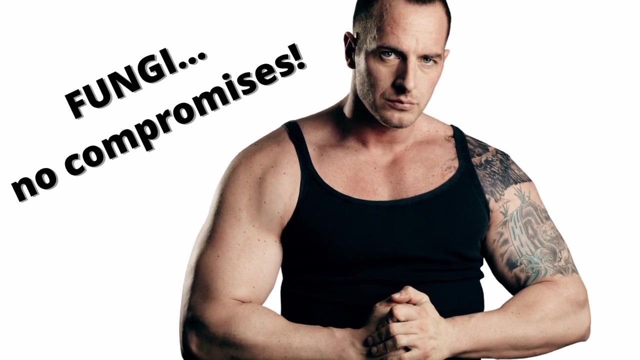 things. but were these things really different? Were they big enough changes? Now, we probably didn't help them that much because our kind of vocabulary was really consistent of telling them to apply fungal dominant compost as a solution And that was kind of it. But actually fungal 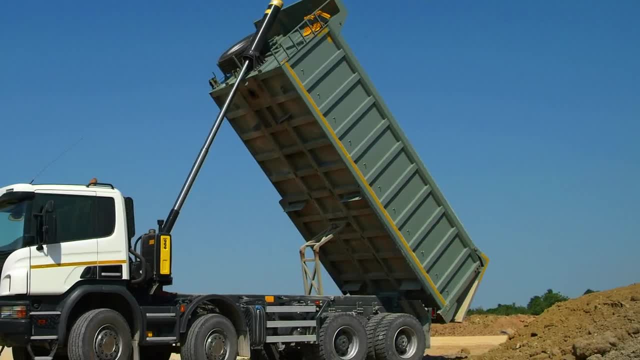 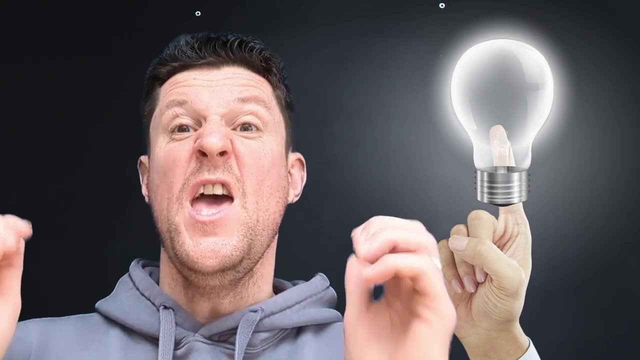 dominant compost is not a good solution. It's not a good solution. It's not a good solution. Isn't really commercially available, So it was kind of a nothing solution. But it took a little while for us before the penny really dropped And we realized what we were doing wrong. or rather, 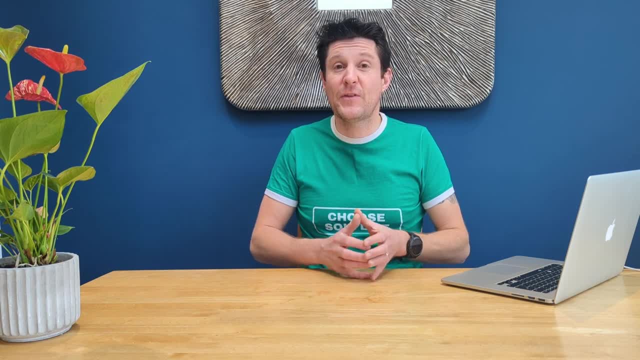 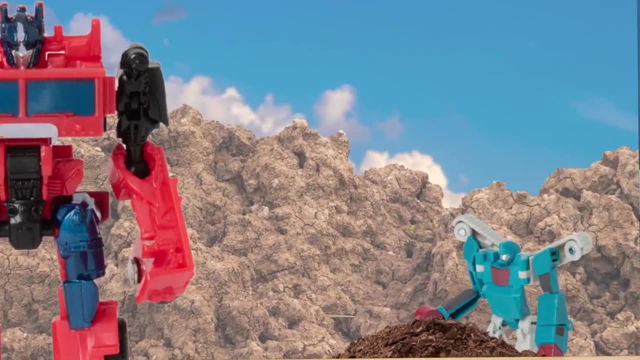 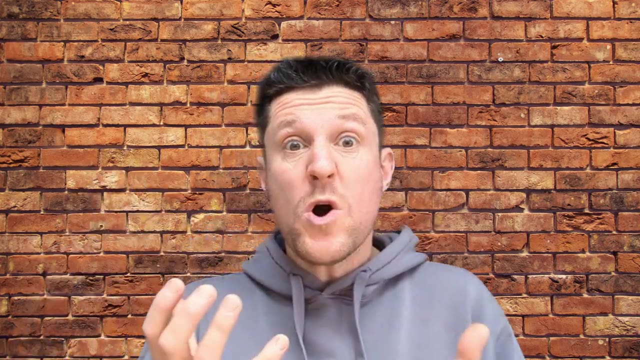 what we were not doing, And we found that there were three principles which absolutely transformed their soil management and boosted their soil fungi through the roof. And what were these three changes that they needed to make? Well, we're going to explore that today. 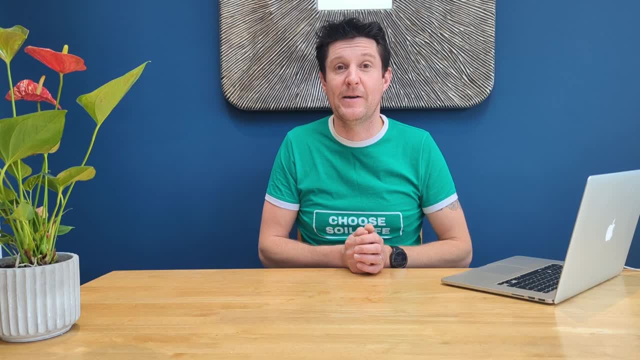 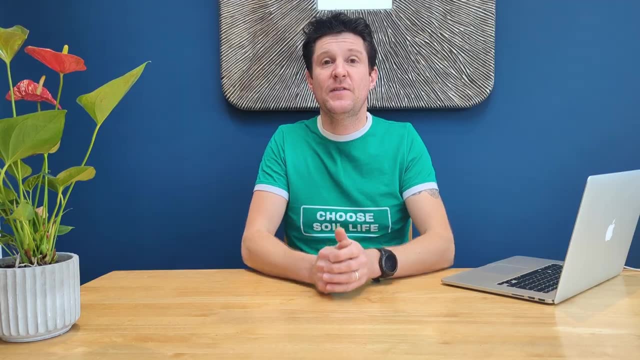 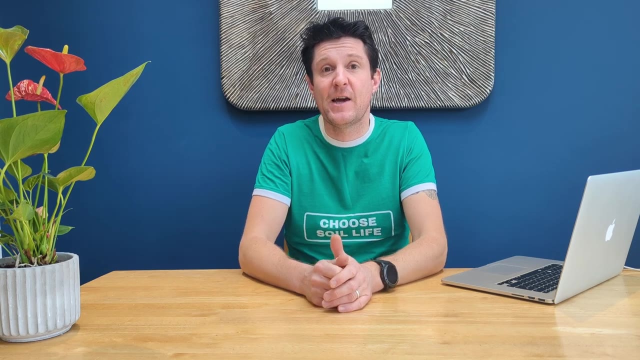 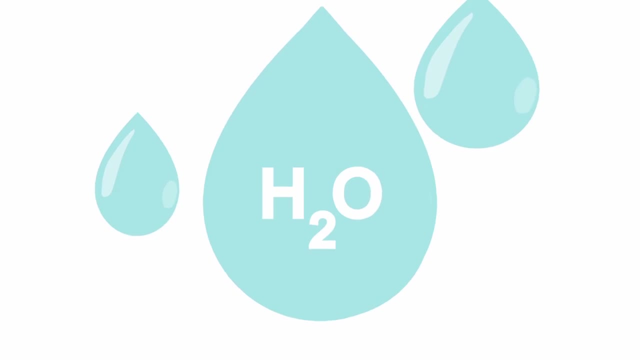 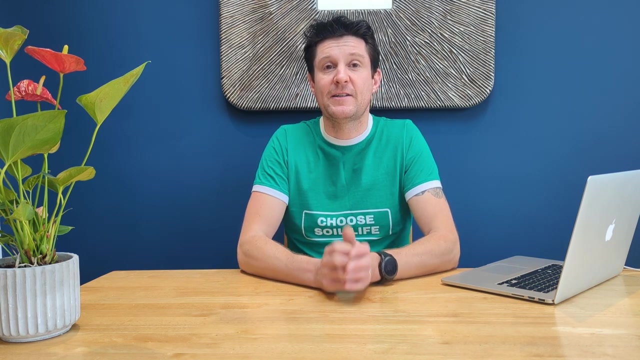 enough oxygen, checking that the water is regulated and controlled- so not too much, not too little- and making sure that There is the right foods available. And making sure that There is the right foods available And, where foods are concerned, what we're talking about for 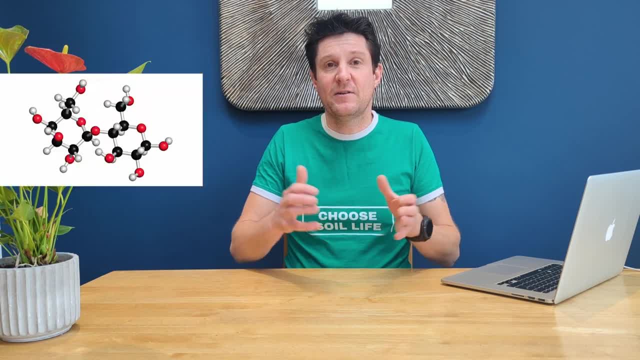 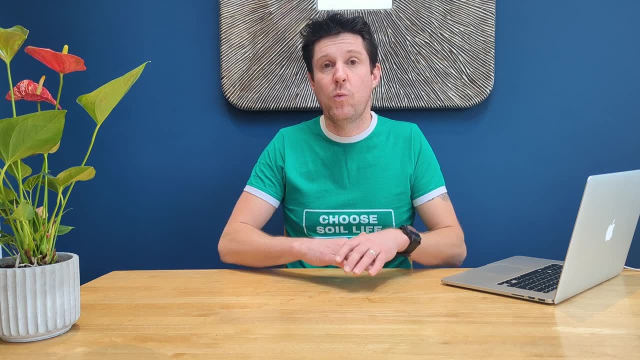 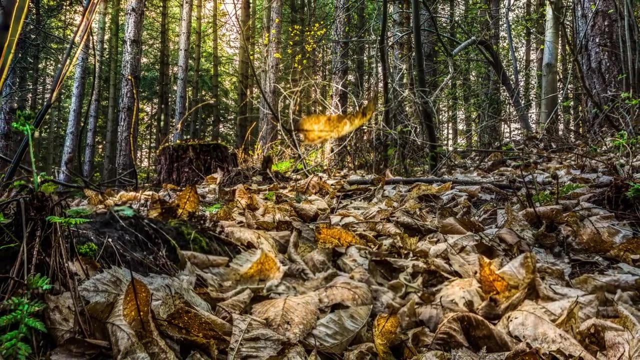 fungi are those complex chains of carbon compounds, the types of food that you find scattered over the floor in a woodland. So we're aiming for a woodland soil and I'm specifically talking about water in easanti woodland floor type effect for our plants and crops. Now, a great way to achieve this is to 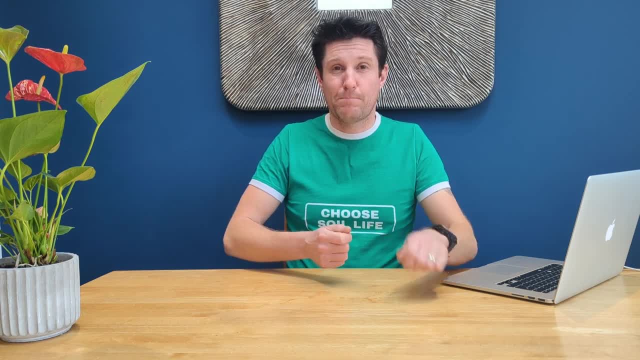 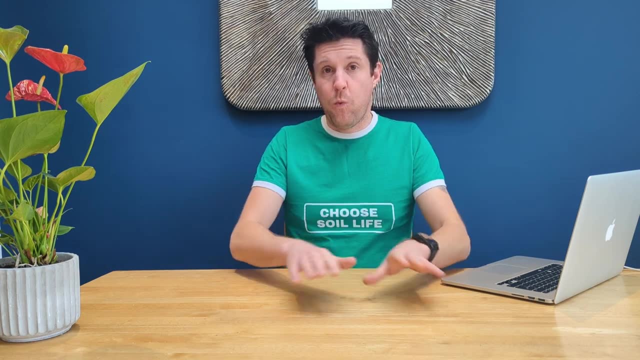 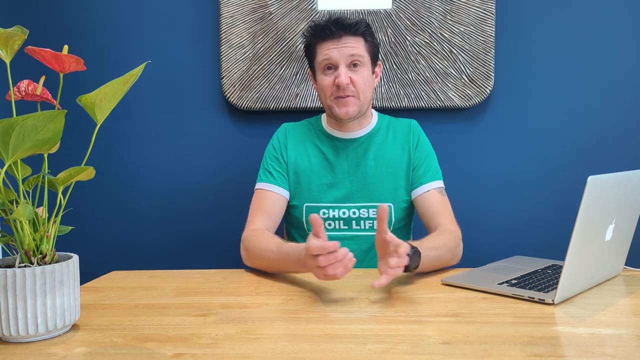 let the bits of leaf litter, twigs, old plants, wood chip- all of these things add to your soil on the surface as one of the foods for what you are growing. And the great thing about this type of system is it's pretty low maintenance. it's certainly low fuss, you just scatter it over. 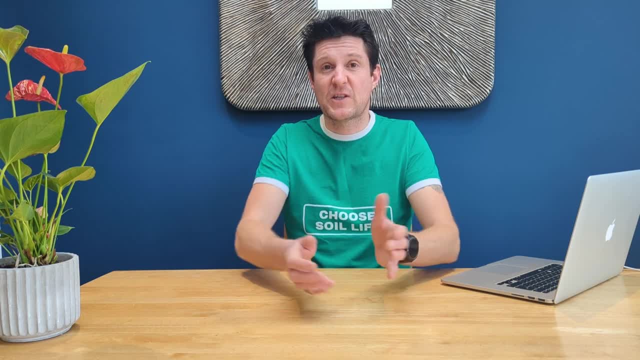 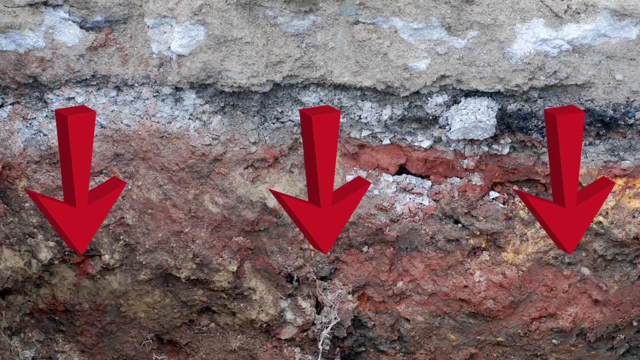 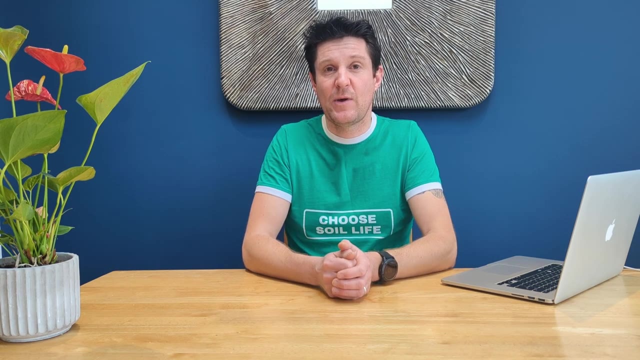 the surface and away you go. Over time it gets integrated into the soil, works its way in and is broken down and turned into foods Along the way. it can also help to retain a little bit of moisture, so it protects the surface of the soil to stop everything evaporating away when it's super. 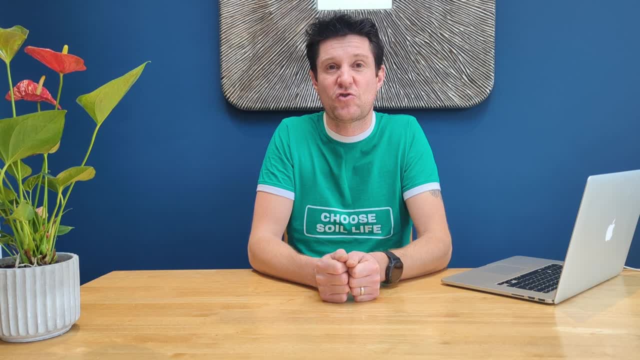 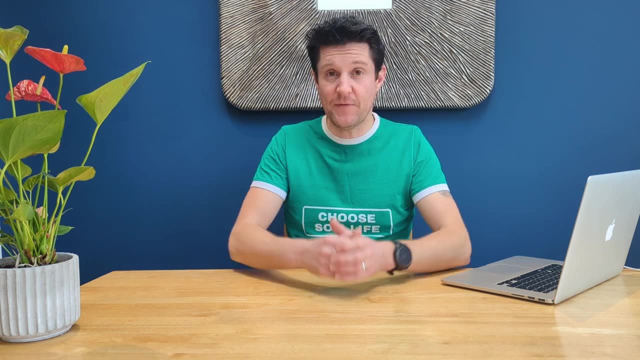 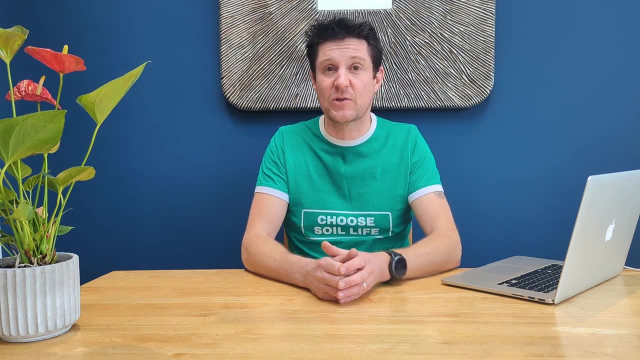 hot. It can also hold onto it in its structure as well and be drawn from also when water is in short supply. The other great thing as well is it's very structural, so as it wheedles its way into the top fraction of your soil, it's adding porosity and structure, so there's more air spaces for your. 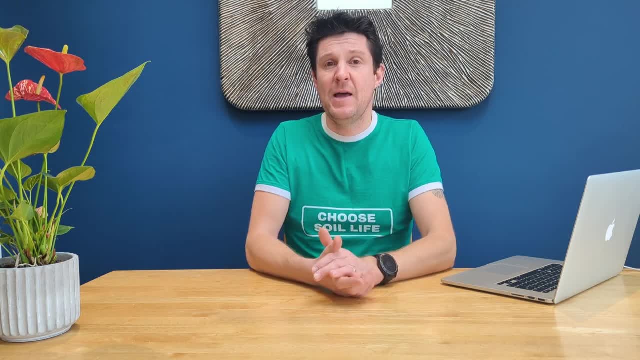 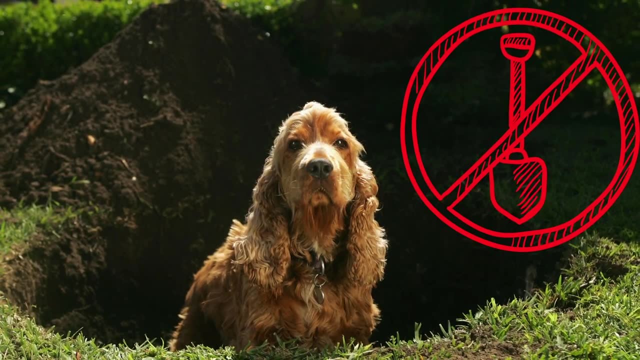 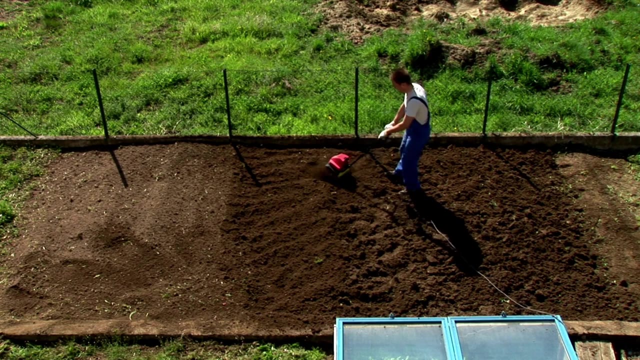 crops as well. But this type of system isn't necessary for everyone unless you're already running no ditches. If you have a big dig where you're used to the surface of your soil looking a little bit different to the classic kind of perfectly manicured billiard table, then you might have problems kind of smashing through that. 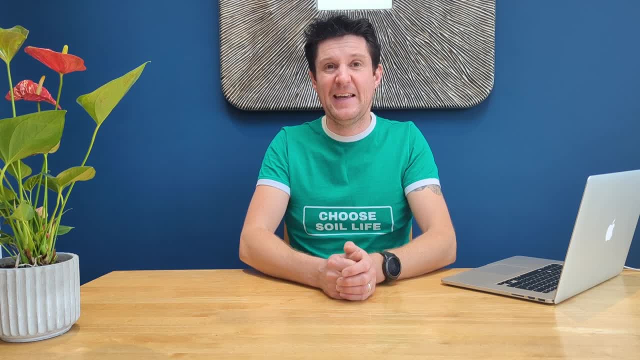 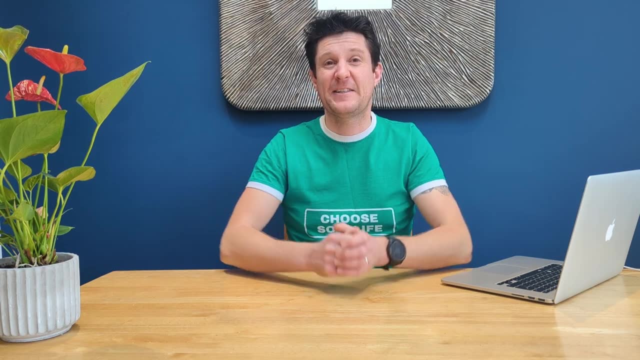 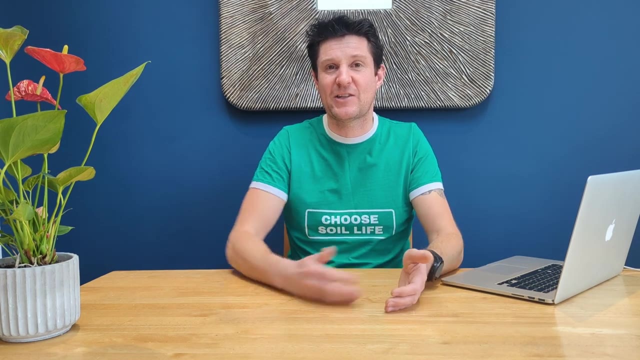 wall and coming over to this way of thinking. It isn't necessarily the most tidy way of growing crops, but it is effective and it is very natural And I think it probably would help you if you do that. So if you're looking to make that transition from really nicely manicured soil to slightly scruffy or more, 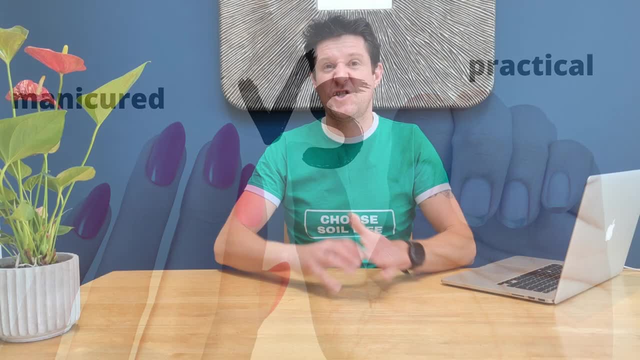 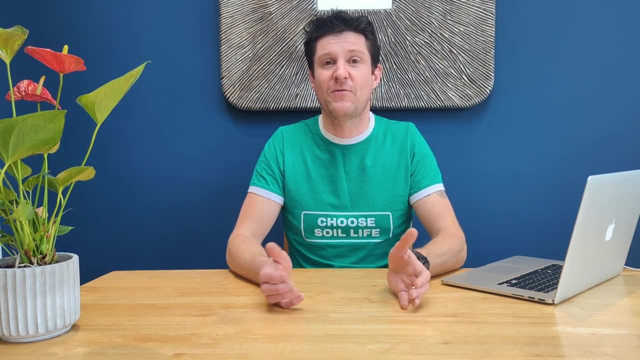 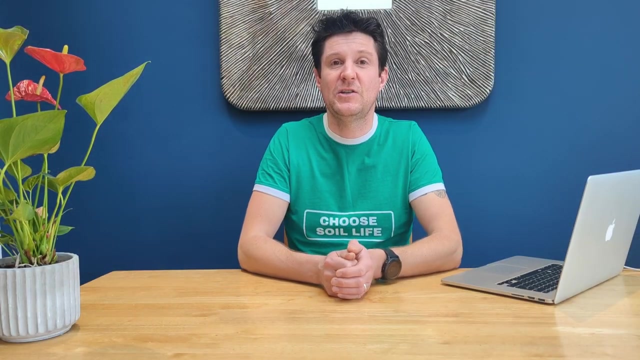 natural. you should be proud of that change to a more natural type of soil environment, One that more closely resembles a forest floor. So woodland floor is the way to go to help ensure that the conditions are right Now. the next great way to boost soil is to use a little bit of soil. So if you've got a little bit of soil in your 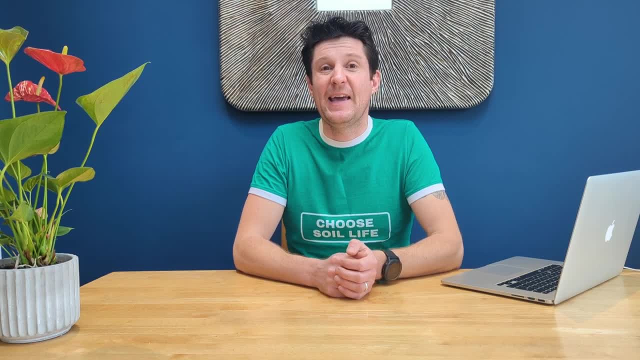 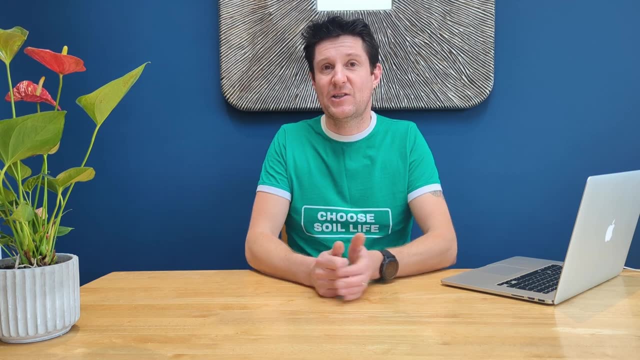 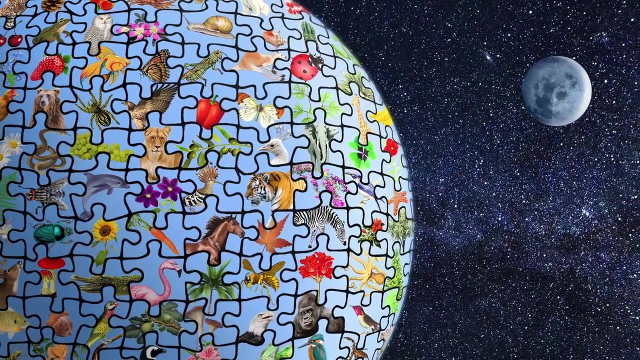 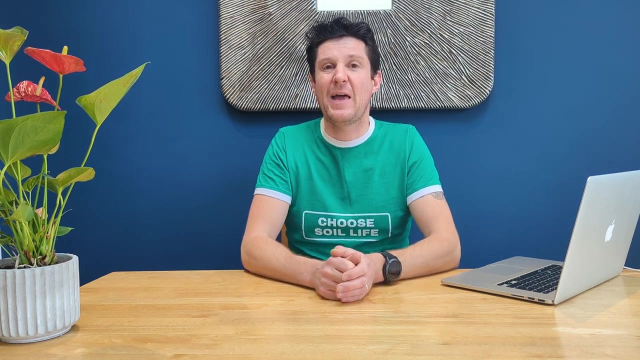 garden, it's a little bit different than if you have a lot of soil. So if you're looking to make that transition from a more natural to more natural soil, then you should be proud of that change. Now a way to do this. well, there's a couple multiple ways to do this. the two main ones are to add a fungal product. 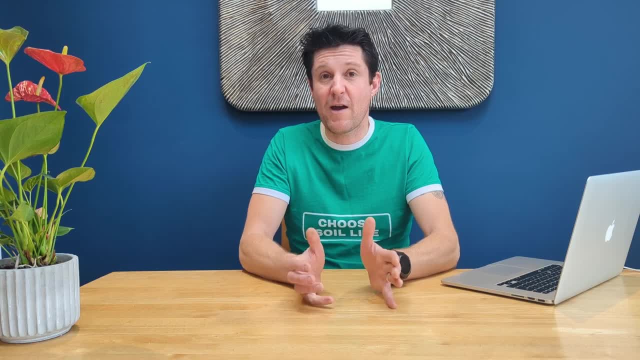 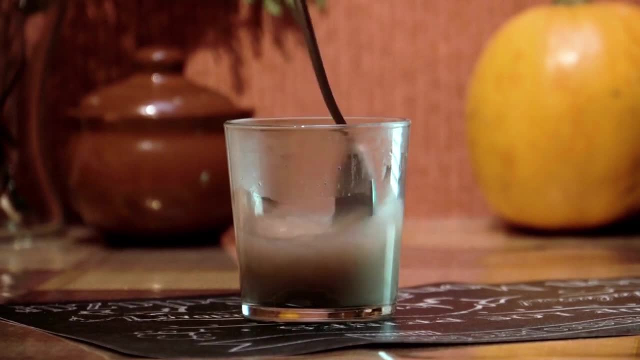 And there's quite a few that are commercially available. They're great to use. They're great to use because they're easy to use. generally, they kind of come in a powder that you mix with water or other materials and apply to your soil. the downside is: 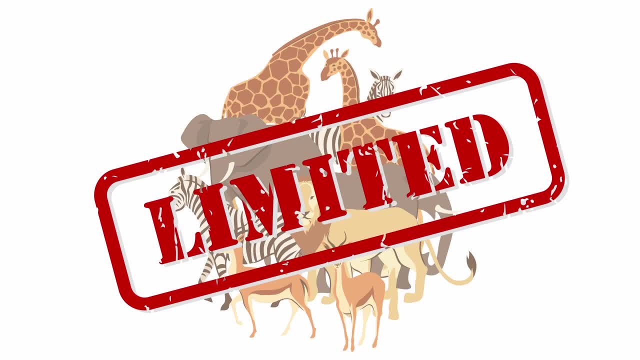 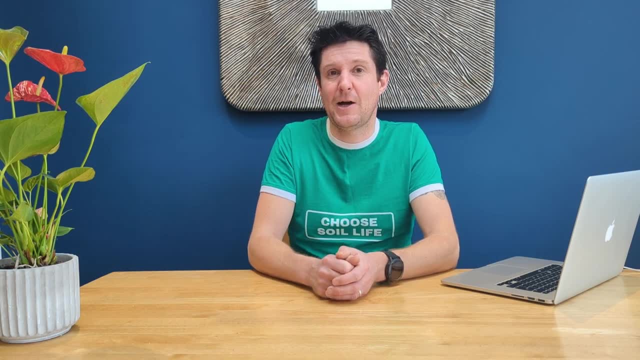 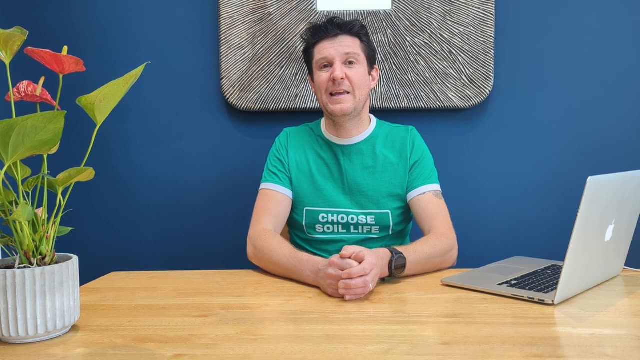 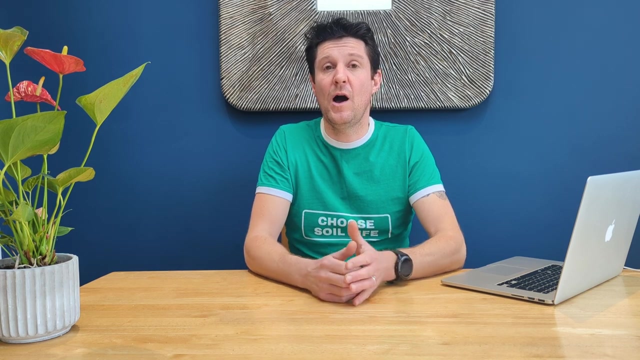 they're often quite limited in terms of the species that they contain, so they tend to kind of Center around the same six to a dozen types of species, so not necessarily the most diverse overall, but highly effective. the other way, of course, to get fungi into your soil is to add your own inoculum, and this could 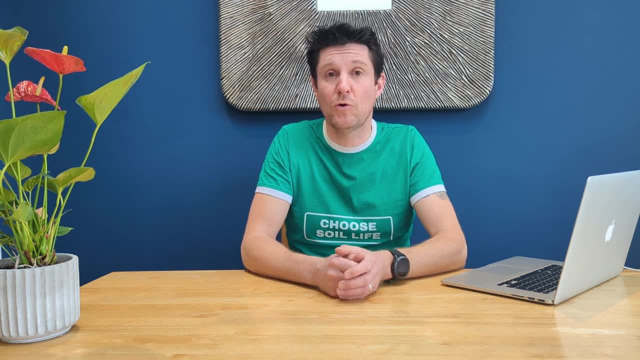 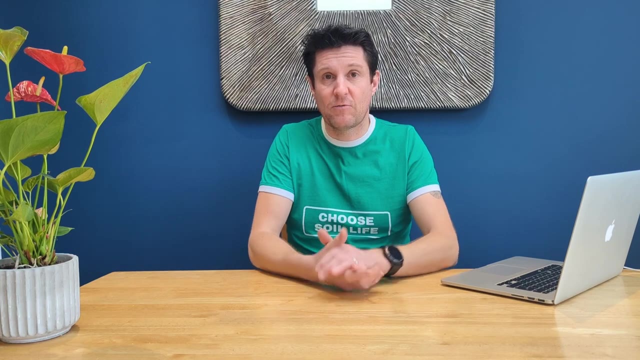 quite simply be a case of taking a small portion of soil from a nearby woodland or ancient woodland, with the owner's permission of course, and you can apply this directly to your soil and all the fungal organisms that it contains with the soil. So if you're looking for a plant that will start to propagate through your soil, or you could mix it. 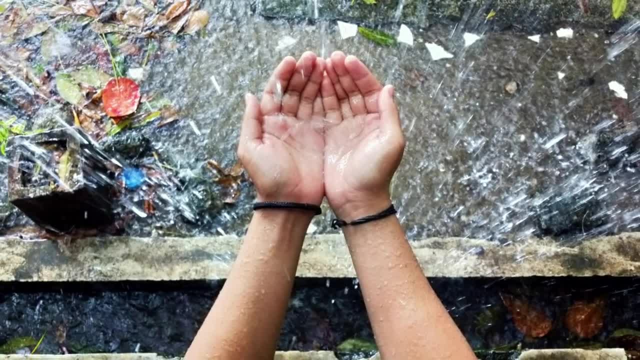 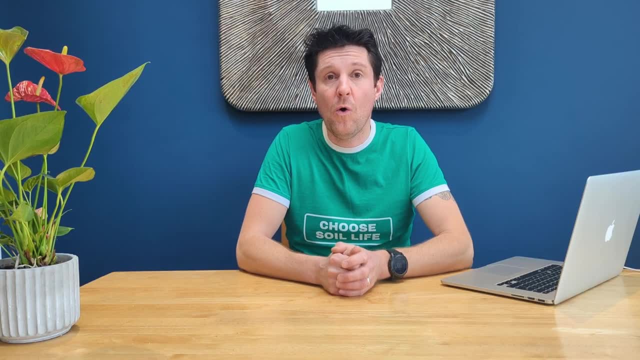 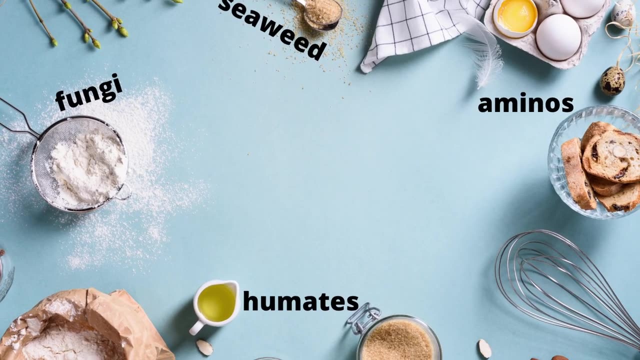 with some rainwater and spread through the soil using your watering can, with the rose on the end, and that's a great way to make it go further as well. or you could make some other kind of amendment or inoculant from it Now, if you think. 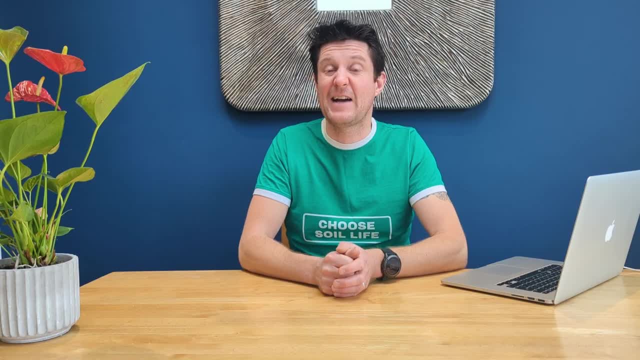 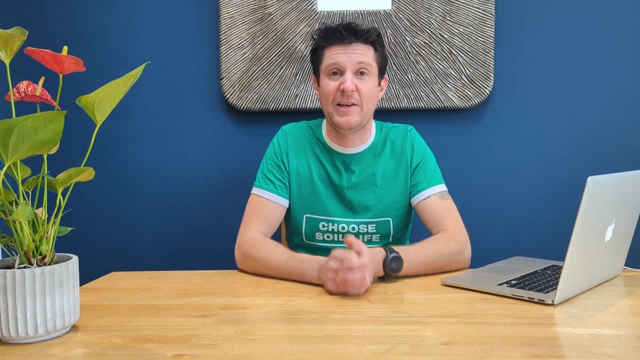 that is the type of thing you're interested in and would like to learn how to do. do. let me know in the comments below. I am- and I'll see you in the next video- Fully up for doing a video on making fungal inoculants, so just let me know. 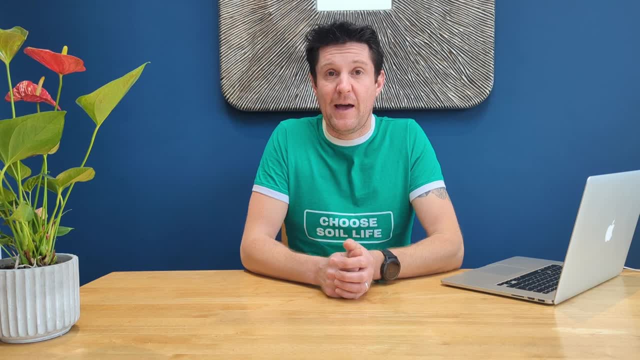 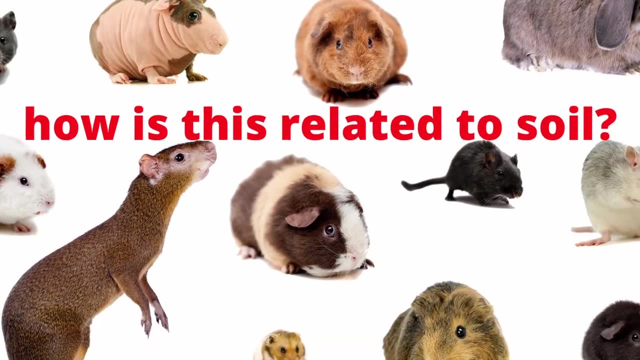 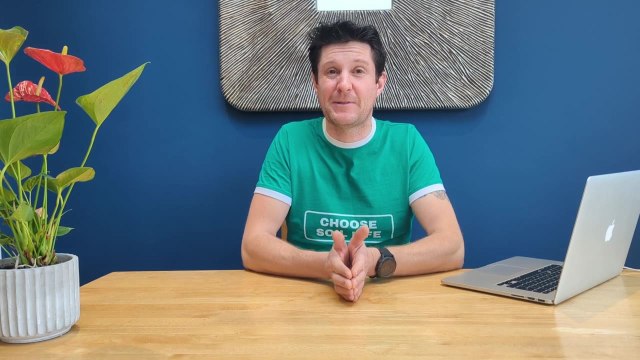 Inoculants are fantastic for not only adding numbers and adding activity to the soil, but they can add different species as well. but it's really quite important when adding species to the soil, to make sure that they are adapted for the soil type and climate that you are in, and that's one of the big issues as well. 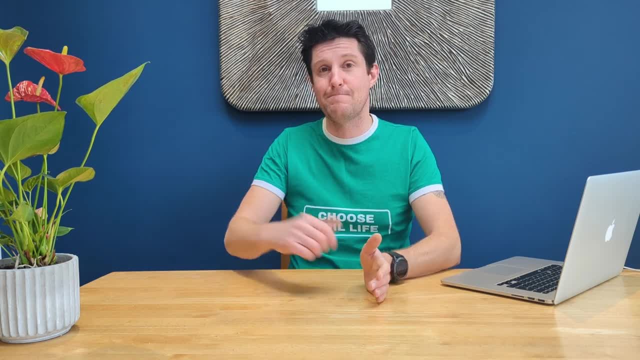 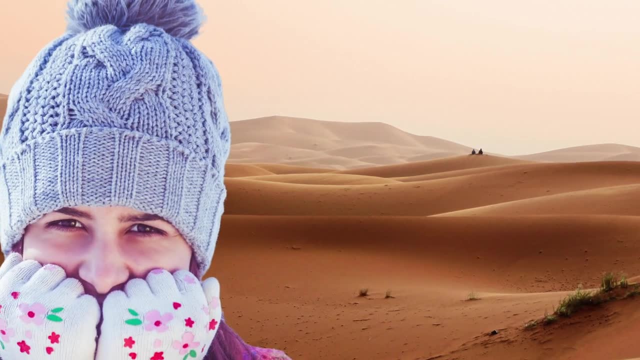 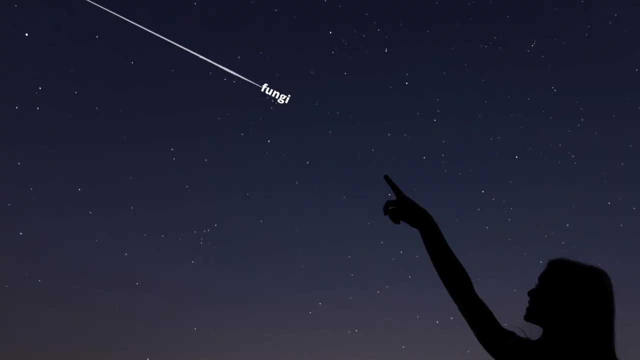 with a lot of the commercial product. if they're made in another country and imported, often the climatic conditions to which they're used, to the temperatures, could be very different to those which ultimately they're going to be used in and in that way the effects, the benefits of them, will possibly be short-lived. so 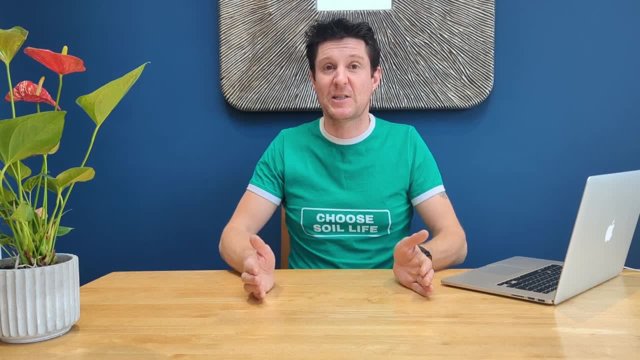 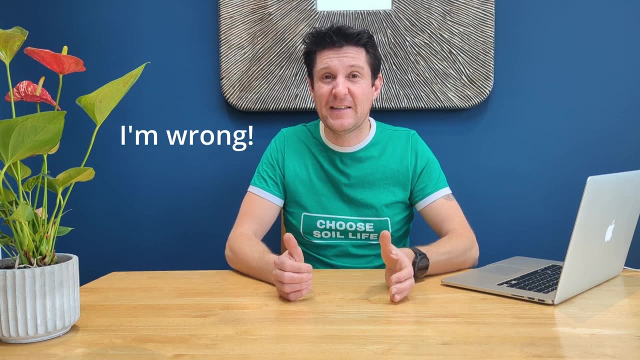 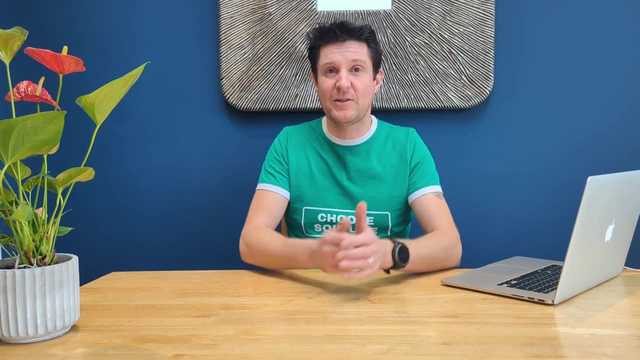 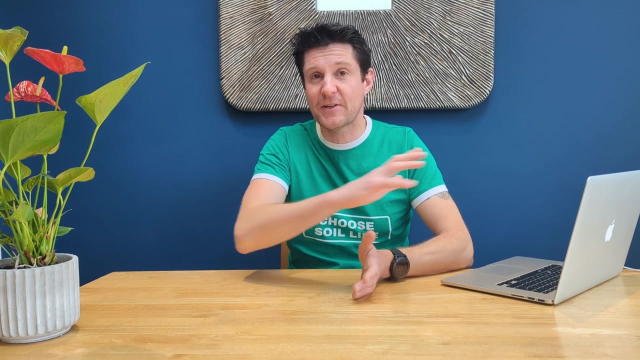 do your research first, try and get as many different species as you can into the soil, and specifically we're looking for endophytes. so those are the organic matter munching types of fungi that will eat up those carbon compounds and convert organic matter into fresh food for our plants. there are other. 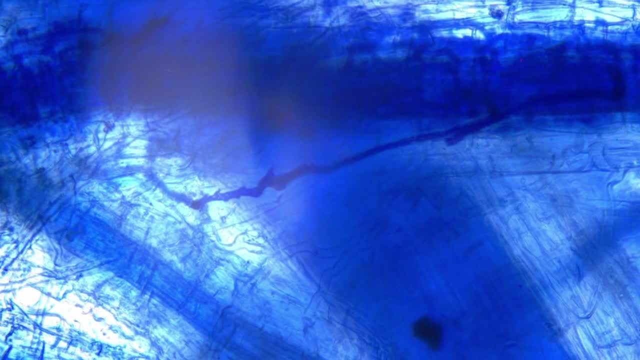 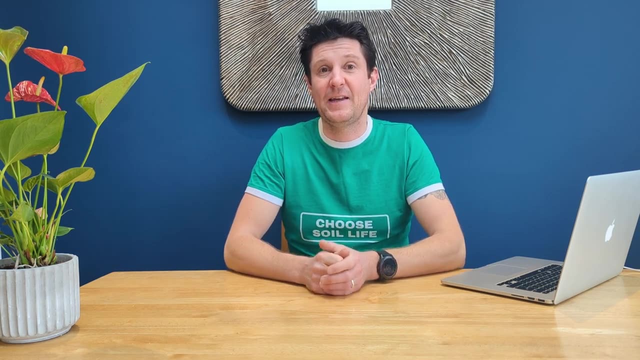 sorts of fungi out there, such as mycorrhizal fungi. that works a little bit differently and perhaps we'll do a video on that another time. one last thing on adding fungal spores and fungal numbers and diversity to your soil. compost tea is possibly one of the most effective ways to make fungal spores. 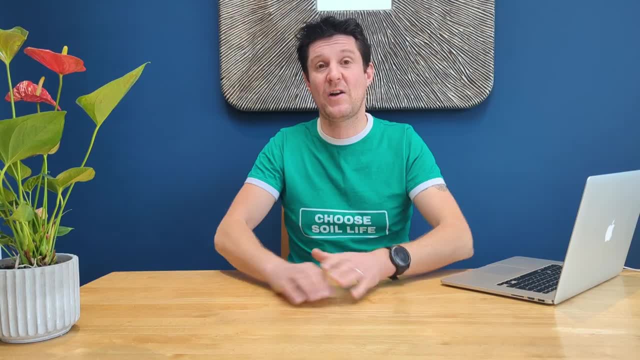 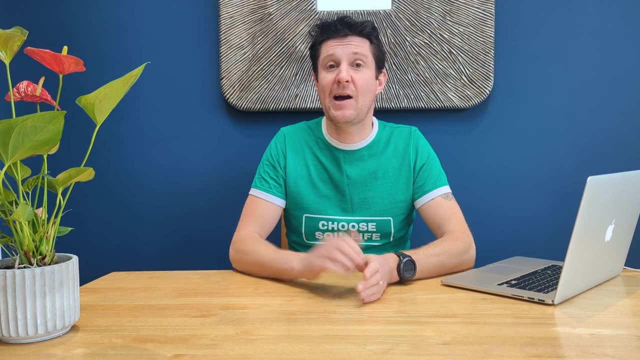 compost tea is possibly one of the most effective ways to make fungal spores worth a look at as well. there are teas, extracts, all kinds of kind of liquid versions of this. if you're interested in exploring that further, then check out one of the other videos I've made as well. I'll leave a link below which: 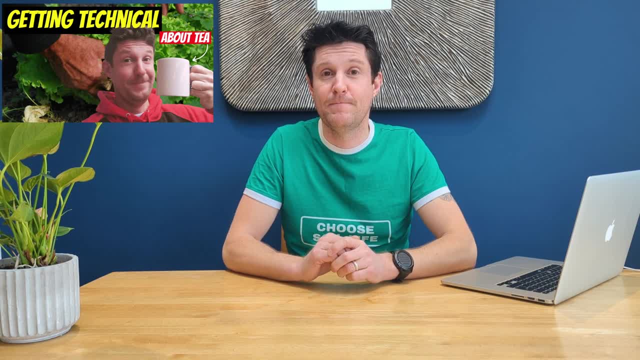 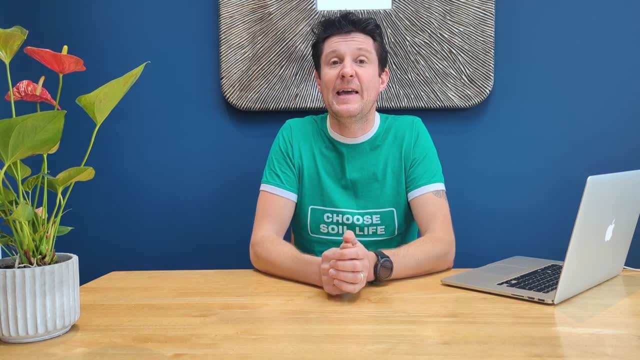 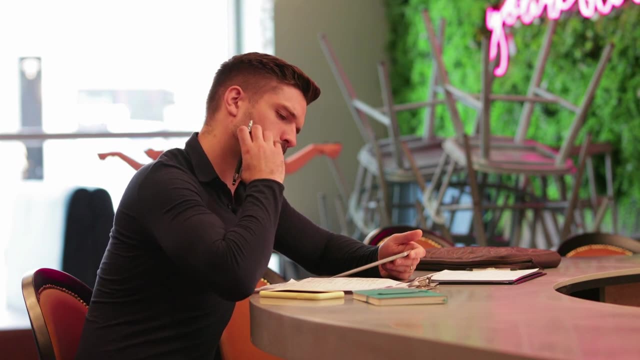 introduces the principles of compost tea. now my third and final principle for you to adopt to drive up your soil fungi is all about crop rotation and planning your cropping. now this should be a principle, if you're serious about growing your own food, that you're already adopting and you tend to plan ahead, thinking about seasonal. 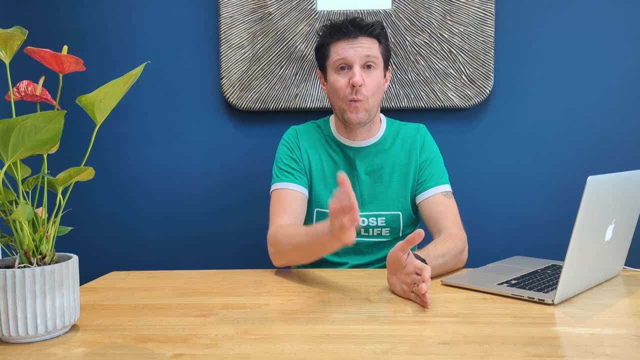 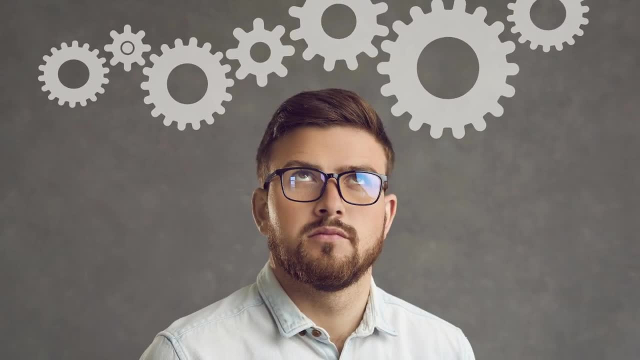 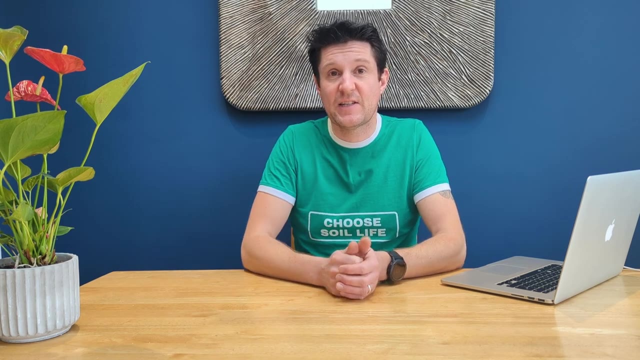 changes and what you would like to harvest and eat, when what I'm talking about here is extending that kind of thought process to include the soil environment as well. now, there are seasonal changes in the soil throughout the year. I've done another video on that, which I'll leave a link to below, which I'll leave a link to below. temperature, humidity and moisture levels affect what's happening in the soil, but what you are growing massively influences this as well. so if you're looking to build soil fungi, you need to consider the very plants that you are growing, and brassicas are a prime example of a type of plant or crop which 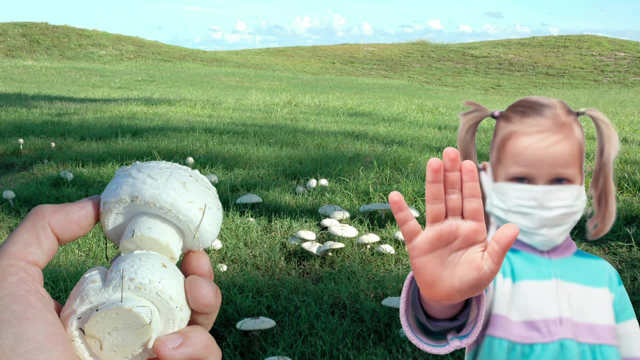 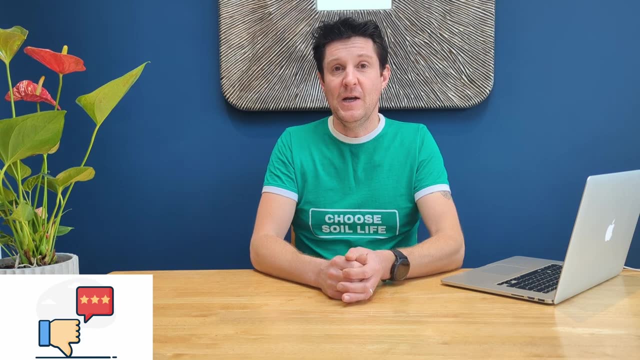 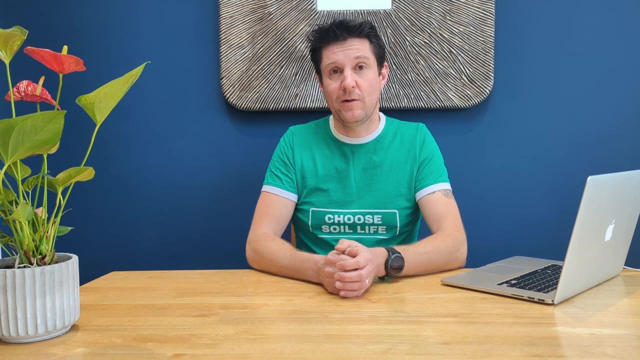 can inhibit fungal development. so if you grow lots of cabbages, this could set back your soil fungi numbers. So the antidote to that is, whenever you're growing something which could negatively impact soil fungi, look to make up for it as quickly as you can. So after your cabbages come out, you want to be planting with another crop which either has no impact or possibly a positive impact, to drive up those fungal numbers as quickly as possible. So all the time you will be affecting the population, the ratio of bacteria to fungi, you want to be returning, if you can, to that equal 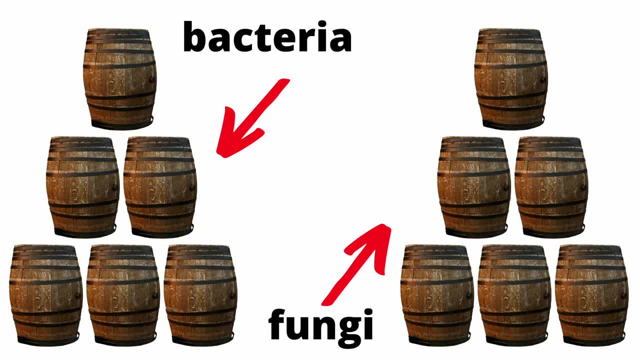 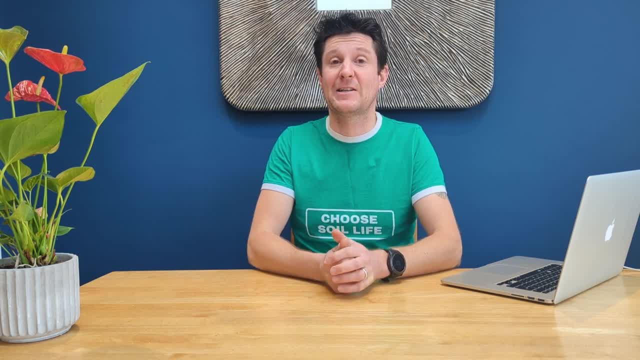 point where you've got an equal amount of bacteria and equal amount of fungi. So plan ahead. think about what you're growing and how that could possibly impact soil fungi and then ways that you could make up for it. An example of mitigating fungal infection is when you're growing something which is not 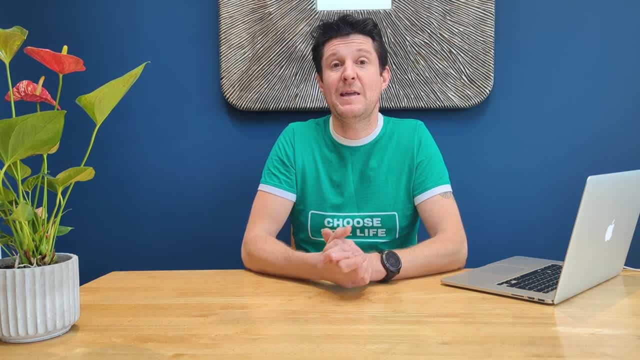 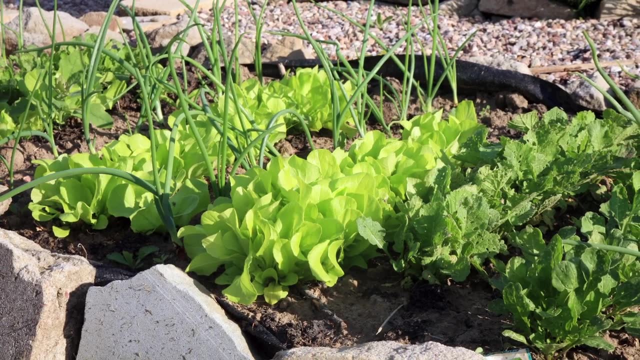 good for negative impacts to soil. fungi Could be intercropping now. years ago, this was adopted by many as a way to manage pests. You could grow a companion crop. something like a marigold next to tomato in a greenhouse is a classic example. You 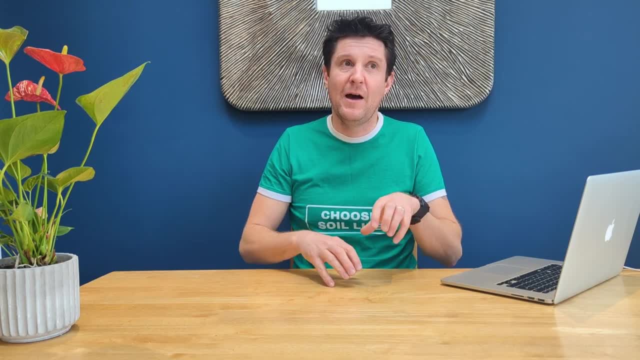 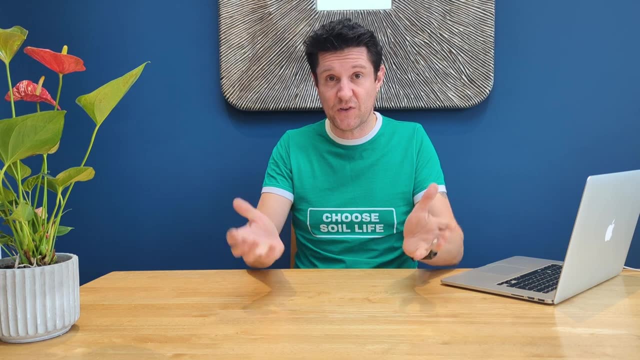 could grow another plant which would either complement or have a beneficial effect for the main cash crop that you are growing. You could think in a similar way with, aside the soil fungus, You could grow something which would either have an effect on the main cash crop you are growing. You could think in a similar way with 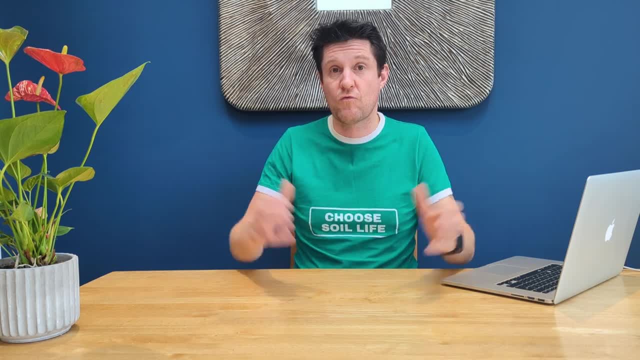 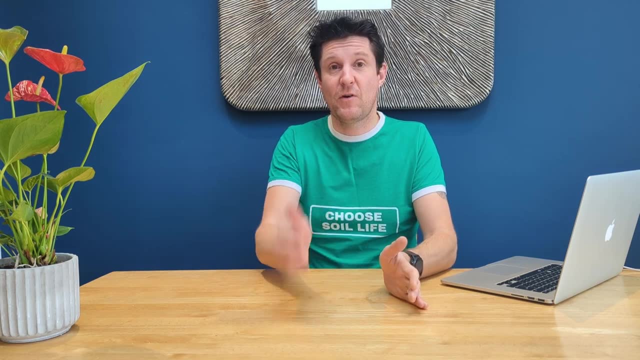 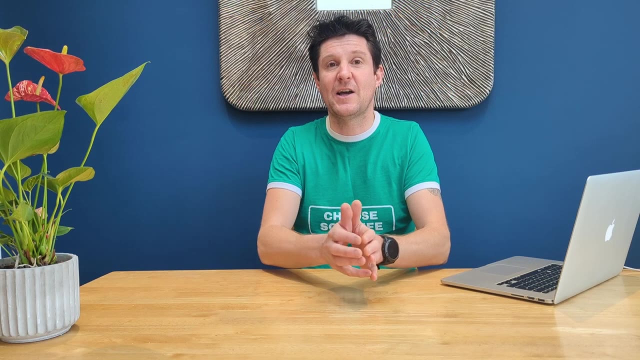 your soil biomass, with the organisms that you're growing underground as well. So if you're growing something which negatively impacts fungi, maybe grow something immediately next to it that positively impacts it, For example, a shrub or woody type plant with cabbages immediately next. 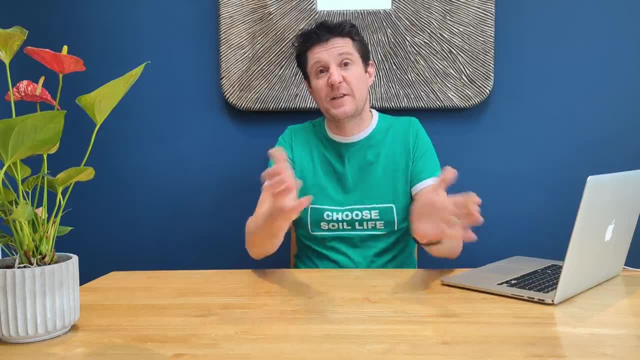 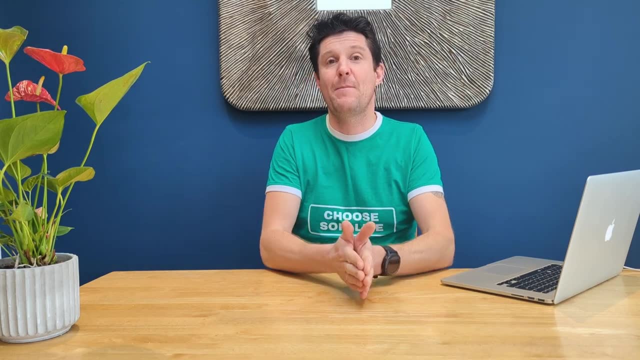 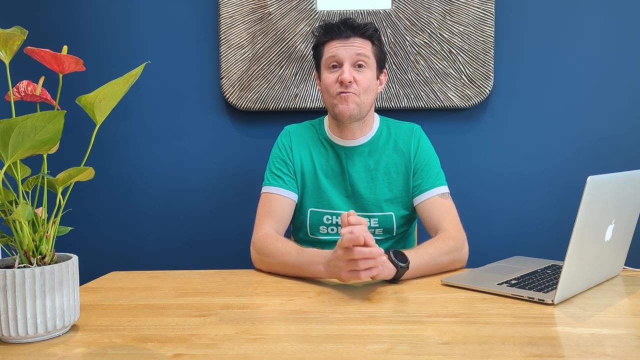 to, it might lessen that impact. Or, if you want to take it to the extreme, you could have an orchard with cabbages planted between all of the trees. You can have some real fun experimenting with this, seeing what works, what doesn't, and you could ultimately end up growing some plants in some